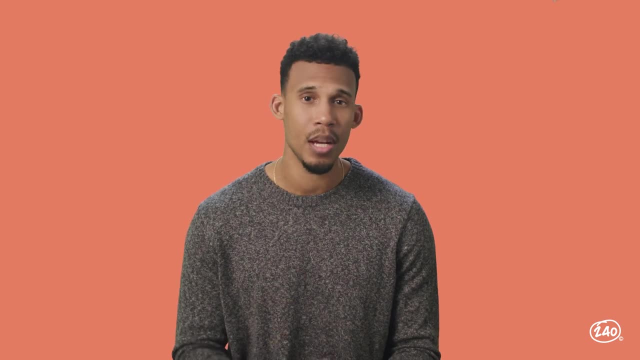 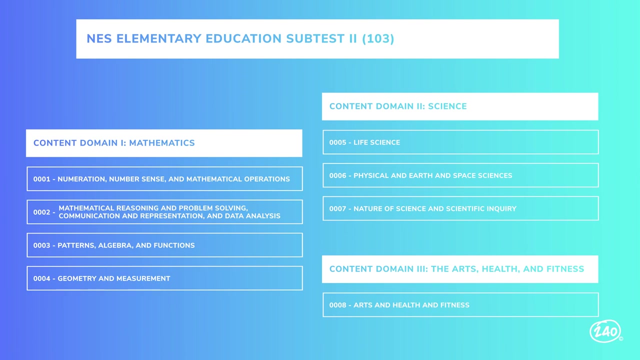 Let's start with each domain. We're going to go over a key concept from each competency Now. these are going to be essential to what you need to know on your exam. Let's start with the biggest domain: math. The first competency is numeration. 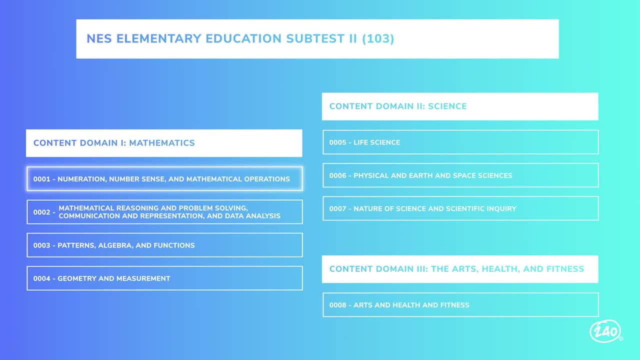 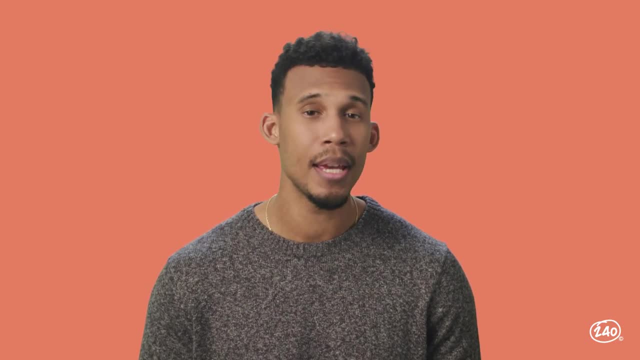 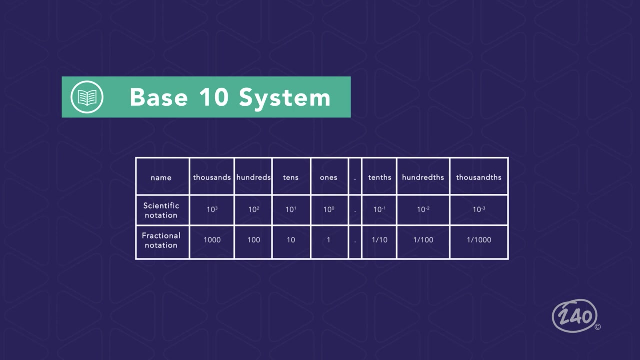 number sense and mathematical operations. This competency covers how students represent and combine numbers. One of the most important things to know for the first competency is place value. That means you'll need to understand a place value chart like this one and the value each digit within a larger number holds. For example, the digit 7 appears in each. 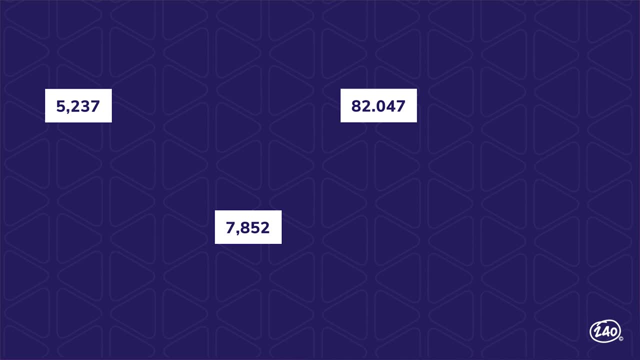 of the three numbers, but it holds a different value in each. In 5,237,, 7 is in the ones place and has a value of 7.. In 7,852,, 7 is in the thousands place and has a value of 7,000.. 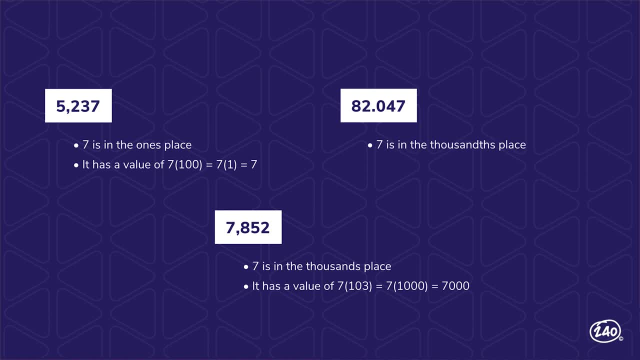 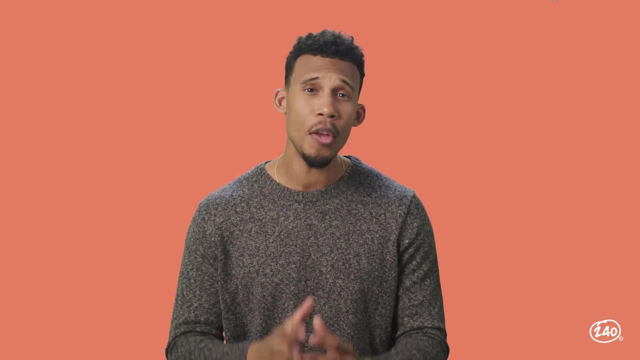 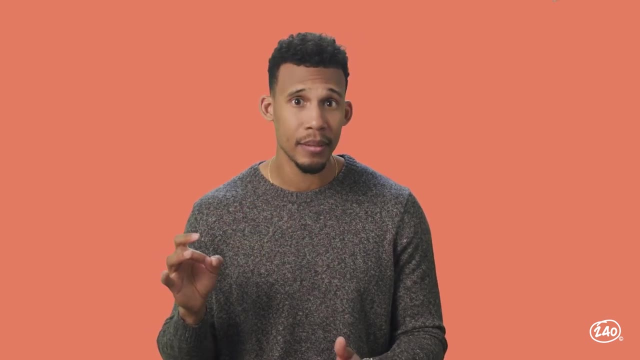 And in 82 and 47 thousandths, 7 is in the thousands place and has a value of point 007.. And here's a tip: Pay super close attention to the ending of these words. It's really easy to make a mistake between thousands and thousandths. 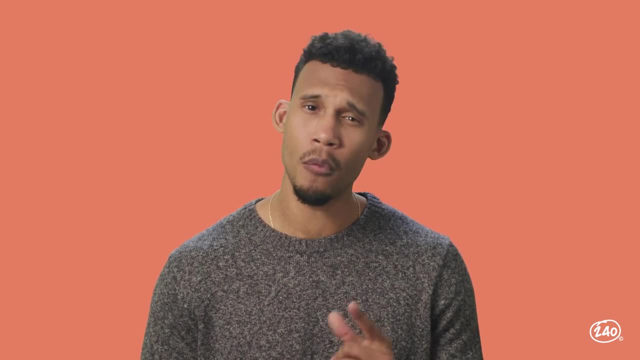 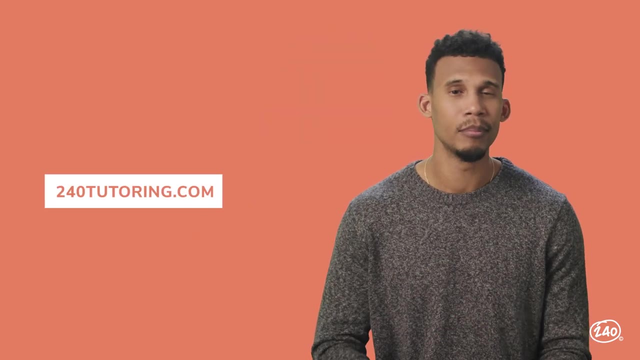 You'll probably be asked to take decimals and turn them into fractions or vice versa, And they may even get a little fancy and throw some percent conversions in. there too Need help with any of that. That's what the 240 study guide is for. 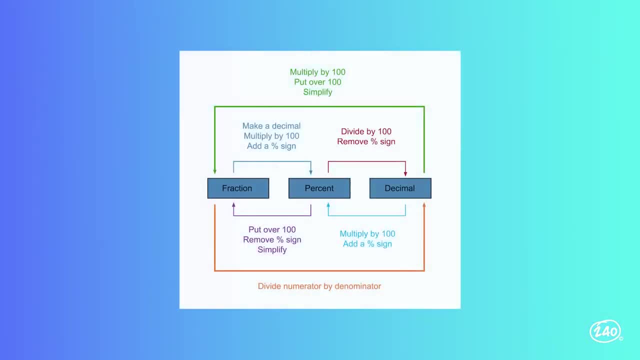 Want me to show you a little sneak peek. I thought so. Here's a handy graphic from the study guide that helps you convert between fractions, percents and decimals. Have a fraction that need a percent. Divide the top number by the bottom. 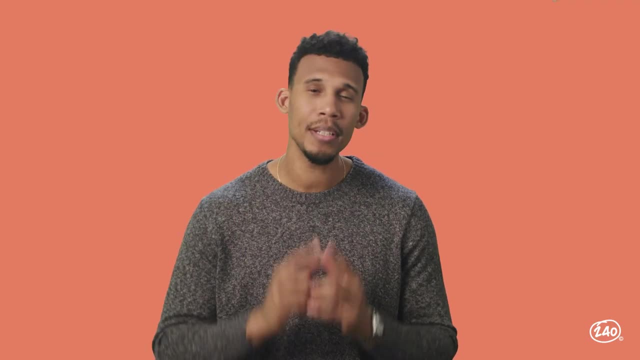 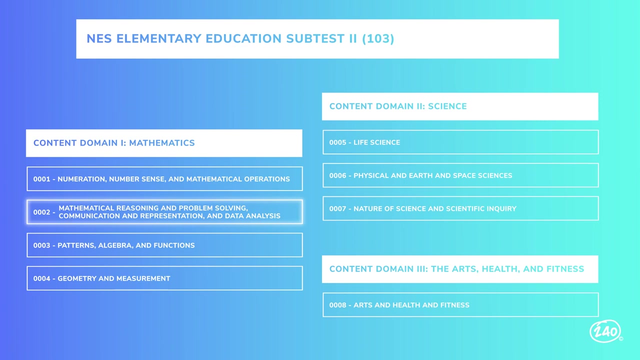 multiply by 100, and add a percent sign, That's one competency down. so let's move on to competency two. Competency two is mathematical reasoning and problem solving, communication and representation and data analysis. There's a lot included in this. 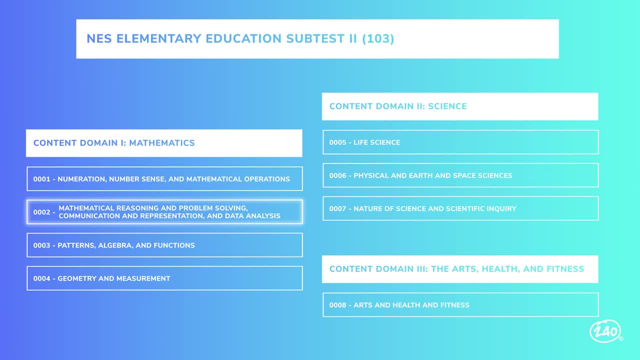 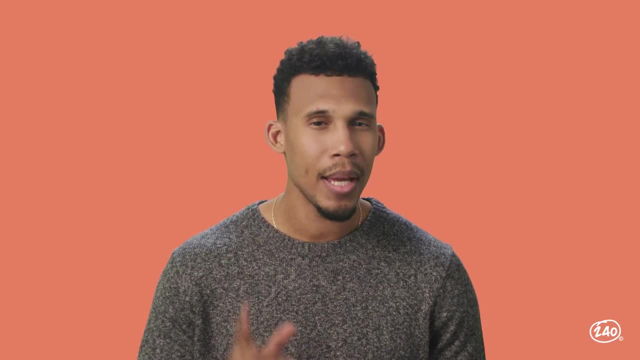 For now, let's get started. For now, let's get started. Now we're going to focus on the data part. You'll likely be given data in a table or chart and asked to interpret it, or you might be asked to do something with the data. 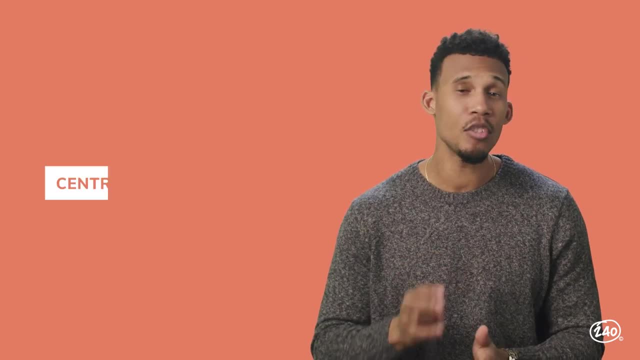 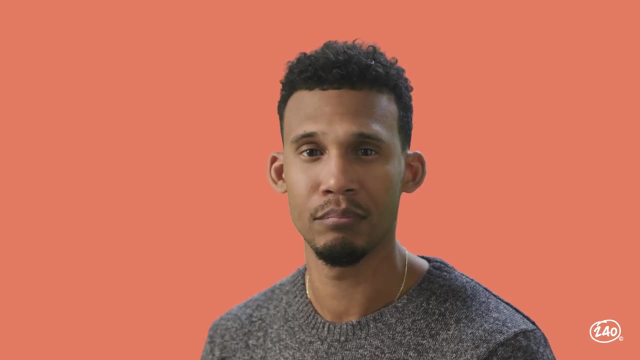 For example, you might be asked to work with the measures of central tendency. They tend to make up a central part of this part of the test. Am I right? Just me? If you're given a data set, you'll need to know how to calculate the mean. 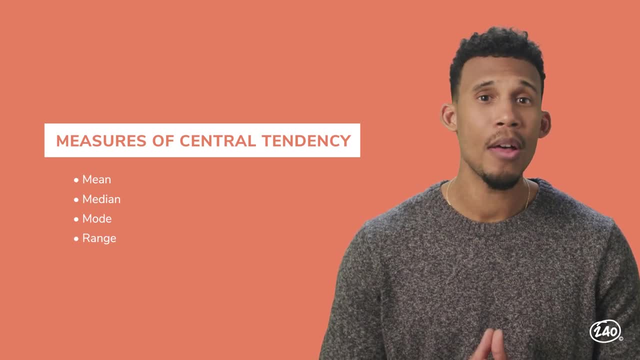 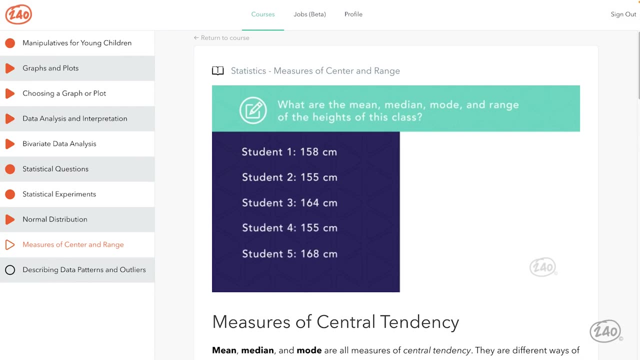 median mode and range. Let's take a look at how these are explained in our study guide. Five students have their heights measured. The data set is 158,, 155,, 164, 155, and 168 centimeters. 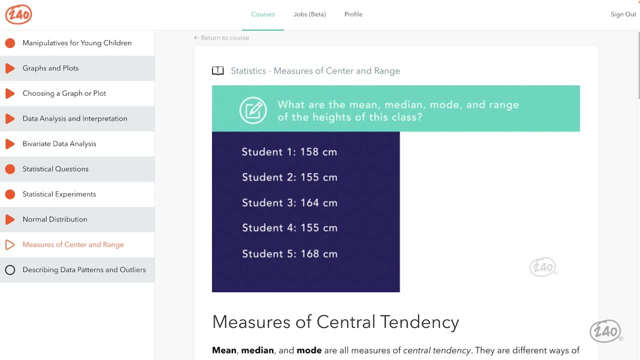 We want to find the mean median mode and range of this data set. First let's rearrange the data to go from least to greatest. We'll get 155,, 155,, 158,, 164, and 168.. 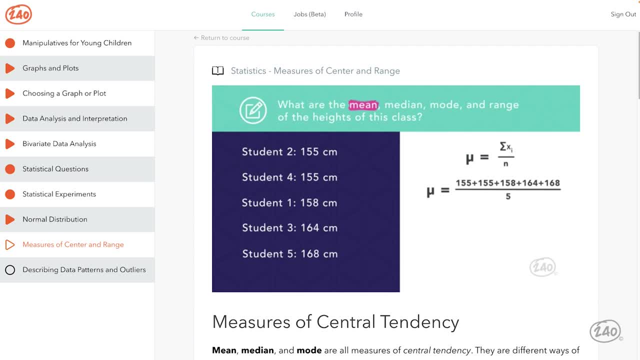 To calculate the mean. we'll need to calculate the mean median mode and range. First add these numbers together to get a total of 800.. Then divide the result by the number of students measured, which is 5.. This gives us a calculated mean of 160.. 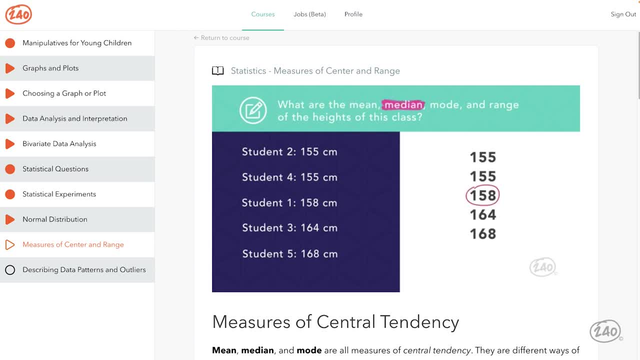 The median is the middle number in our organized data set, which is 158.. The mode is the most frequent number, which here is 155.. And our range is equal to 168, the highest number minus 155, the smallest, which equals 13.. 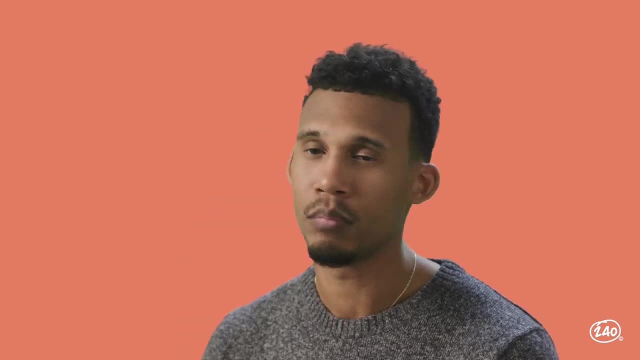 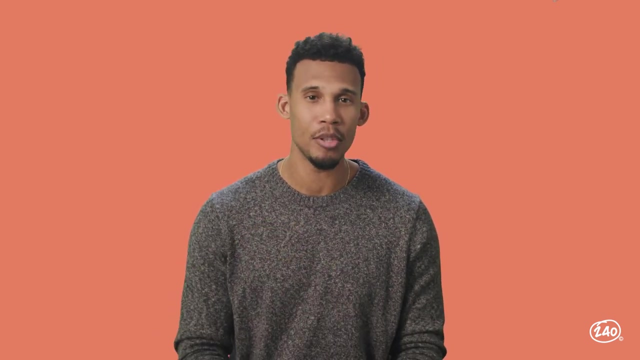 Are you starting to feel like these skills are in your range? No, Okay, fine, I get it. You hear from my brilliant testing knowledge, not my terrible jokes. In that case, let's move on to competency three. The third competency in domain one. 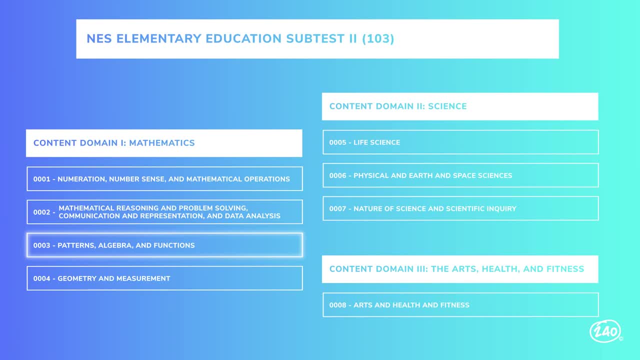 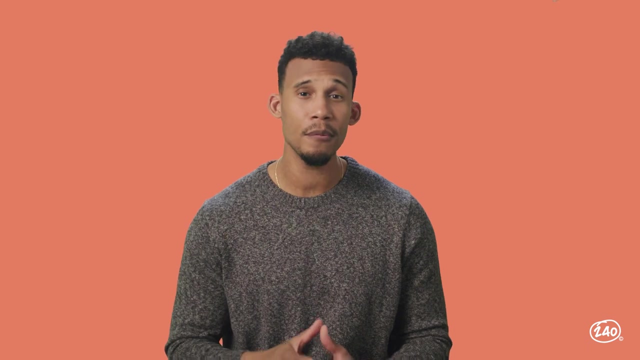 is patterns, algebra and functions. This covers recognizing patterns in number sequences and using your understanding of patterns to make predictions. You'll also need to recognize functions and use algebra to solve real-world problems. Since there are two mentions of patterns in the description for this competency, let's focus there. 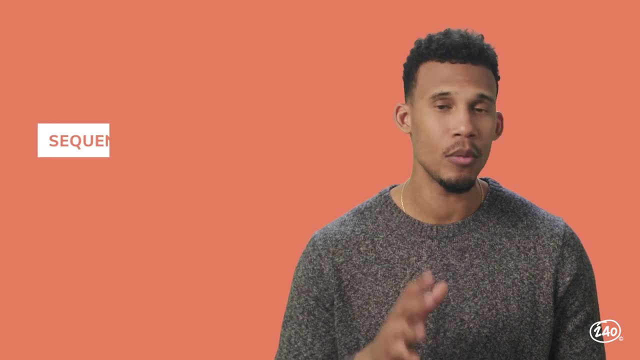 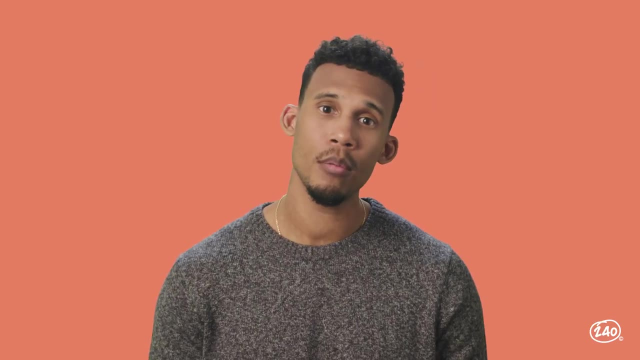 Another, more math-specific name for a pattern is a sequence. A sequence is a list of numbers, shapes or symbols that go in a specific order. So in general we're looking at three types of sequences here. First up, you've got arithmetic sequences. 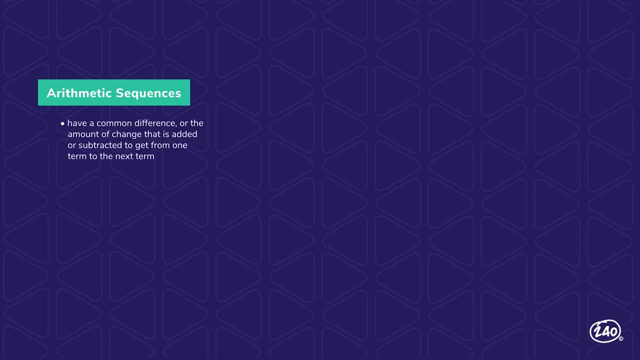 and these are usually the easiest to figure out. They have a common difference between terms Meaning. you add or subtract the same number every time you go from one term to the next. In this example, we add five to get from one term to the next. 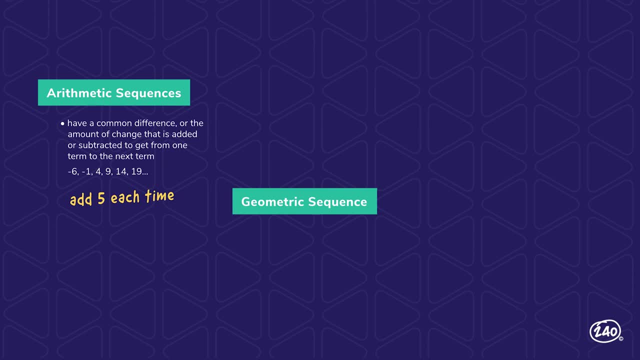 Then you've got geometric sequences. These are a little trickier, but you can handle it. In these you need to either multiply or divide by the same number to go from one term to the next. In this example, you multiply by three each time. 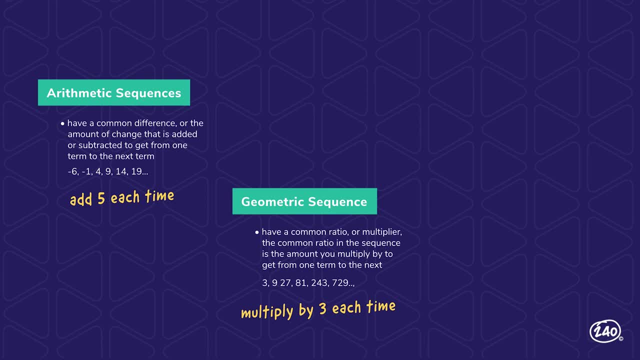 And then you've got the trickiest one, and I think that we're trying to be funny because I even named them: complex patterns. In a complex pattern, you're going to have to identify two separate patterns. So, looking at the number sequence: 6, 2,, 7,, 3,, 8,. 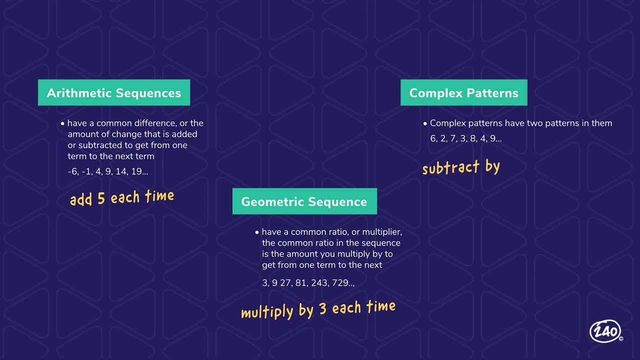 and so on. to go from 6 to 2, you have to subtract by 4.. Then when we go up to 7, you need to add 5.. And you go back and forth between these two actions: Subtract 4,, add 5,, subtract 4, and so on. 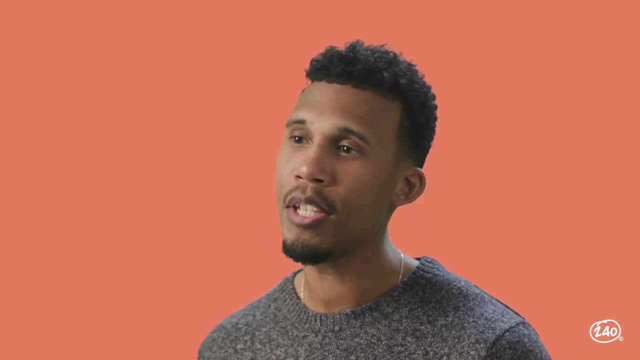 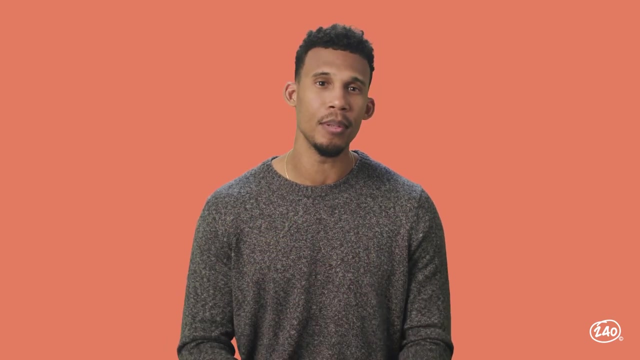 Now, that's just one piece of this competence: To see everything you need to know to be successful on the test, subscribe to the study guide. Are you guys ready to move on to competency four? Let's do it. The fourth competency is geometry and measurement. 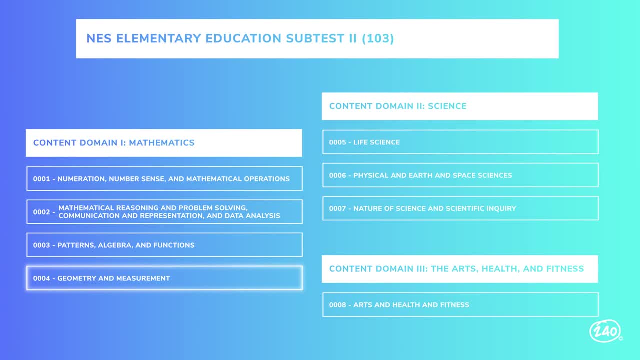 It covers a basic understanding of shapes and how they relate to each other, So you'll see things like similar and congruent shapes and how to calculate area and perimeter. It also covers using appropriate measuring tools and converting between measurement systems. There's a lot to unpack in this one. 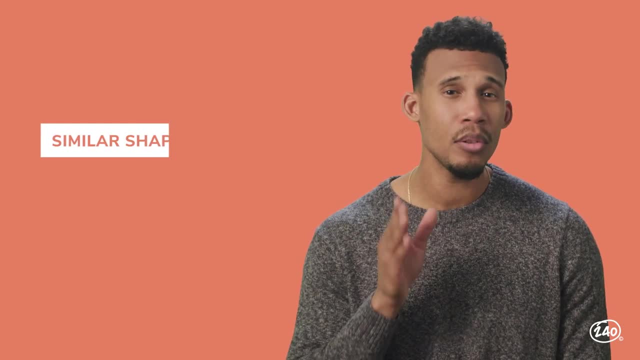 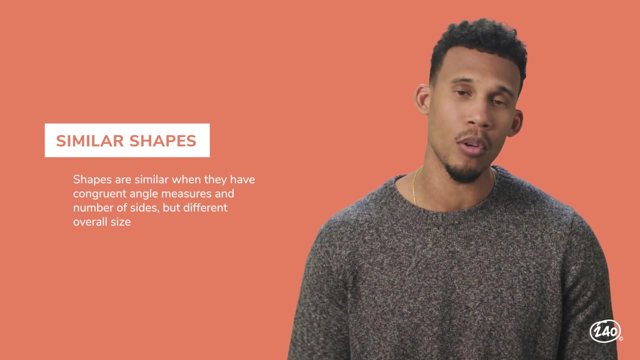 but one thing you're likely to find and you're likely to see on the exam is similar shapes. Shapes are similar when they have congruent angle measures and number of sides, but different overall size. When shapes are similar, you can relate them to each other. 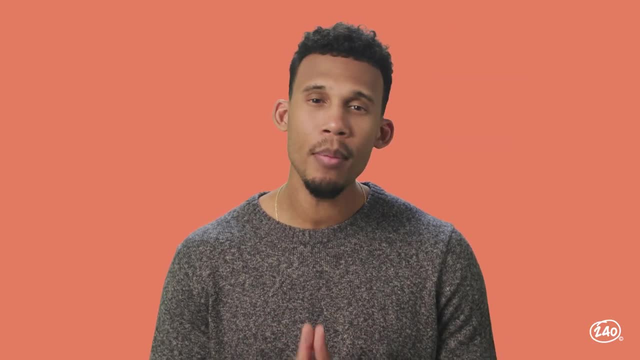 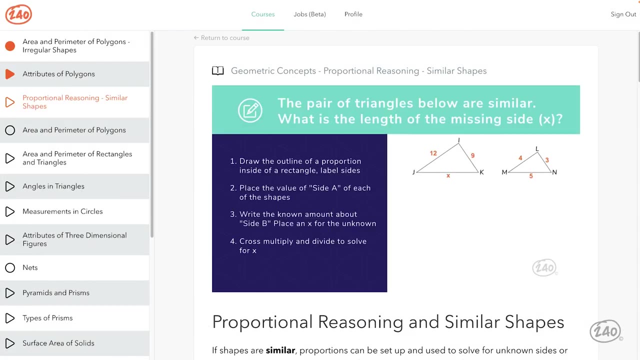 in order to find missing side lengths. Now, I know you probably want to see an example of this, right, So let's head over to the study guide. The two triangles here are similar. Let's find the length of the missing side x. 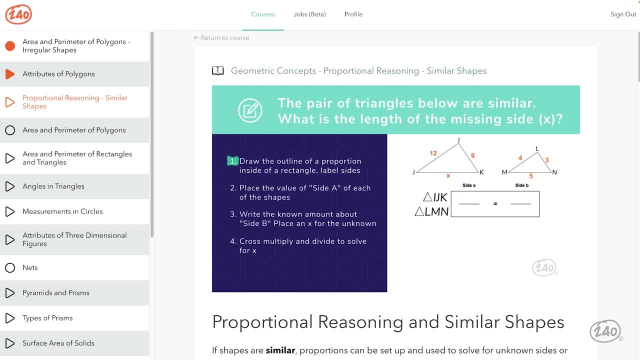 First we'll draw the outline of a proportionate triangle. Let's draw the outline of a proportion, two equal fractions inside of a rectangle Label. the left side of the rectangle, with two different shapes On the top of the rectangle label. the first fraction, side A. 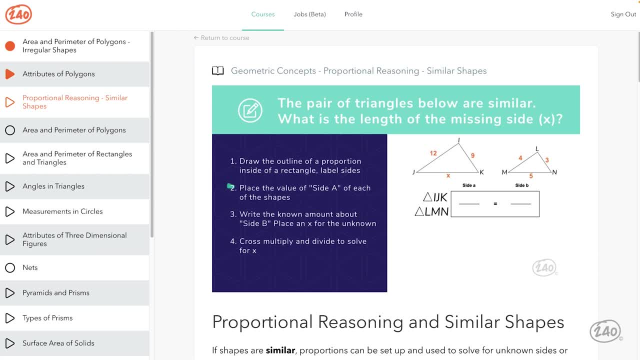 and the second fraction, side B. In the first fraction, place the value of side A of each of the shapes, making sure the labels to the left correspond appropriately. In the second fraction, write the known amount of side B, Then place an x for the unknown amount. 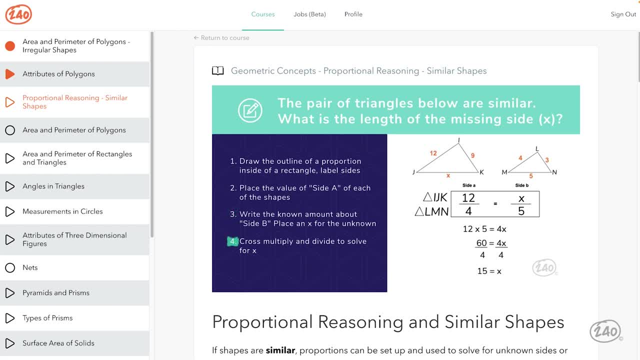 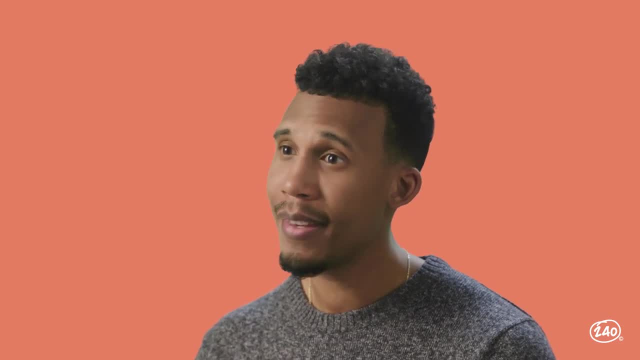 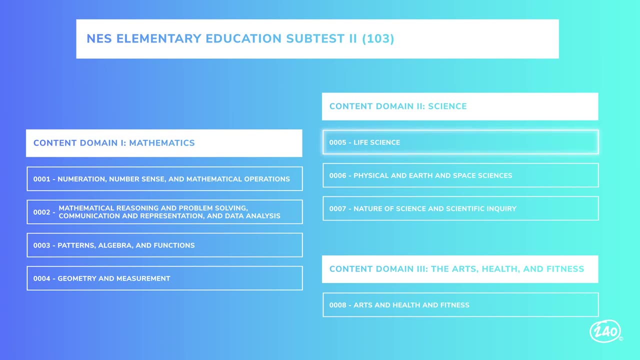 Then once again cross, multiply and divide to solve for x, Like what you saw. There's a ton more videos where that came from. We finished math. Now let's head over to science. The first competency in science is life science, So you're going to need to know the characteristics. 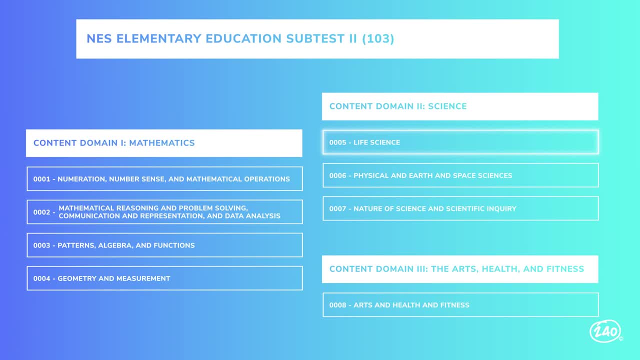 and life processes of different organisms and how to classify them. You're also going to need to know how they reproduce, what their life cycles are and how to classify them. You're also going to need to know what life cycles look like and how they interact with the environment. 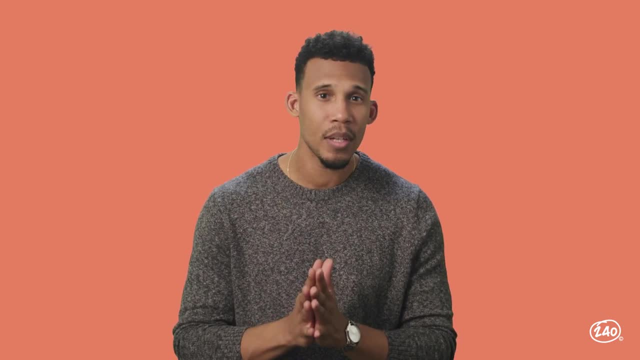 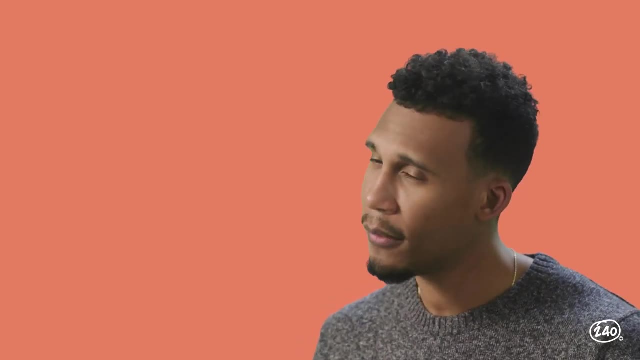 That's not a lot. right Now, I know that's a lot. That's okay, because we're going to pinpoint one of these and zoom in on it. Let's dive into characteristics of organisms, specifically adaptations, which are the traits that improve functions. 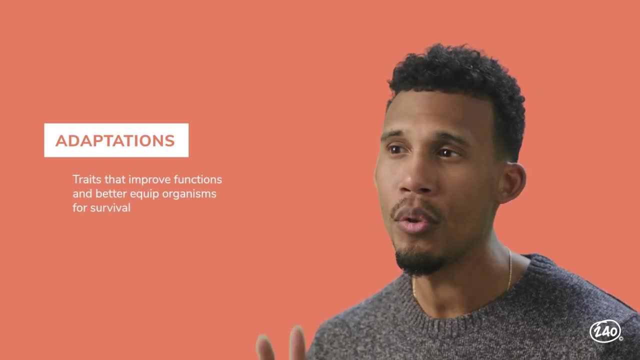 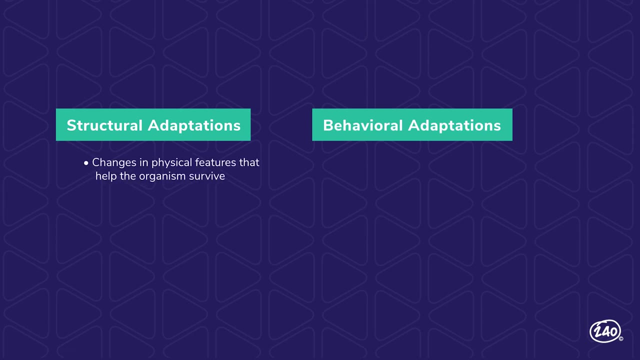 and better equip organisms for survival. There are two types of adaptations an organism can have: structural and behavioral. Structural adaptations are physical features that help an organism survive. Think a bird species that develops a different beak shape that makes it easier to get food. 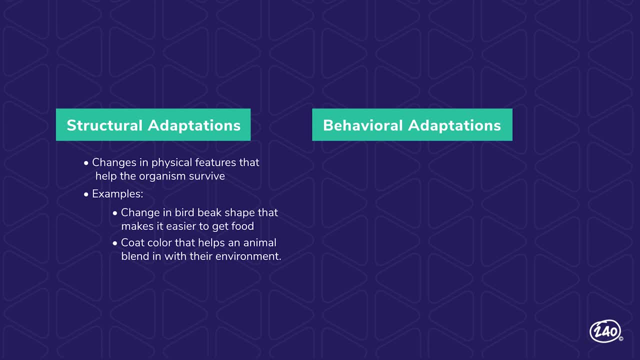 or a coat color that helps an animal blend in with their environment. Behavior adaptations are things that organisms do naturally, usually to avoid harm, like when a skunk sprays scent for protection or a bird migrates to avoid cold temperatures. And if you need a little more help with this, 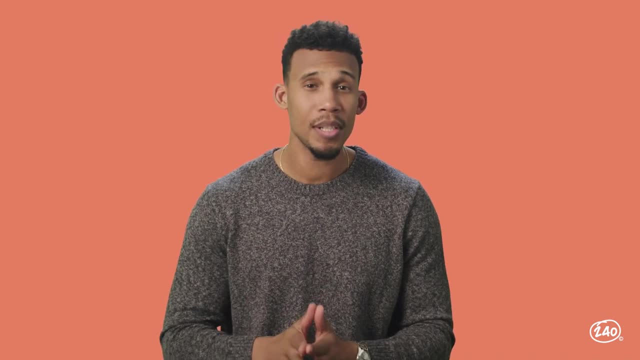 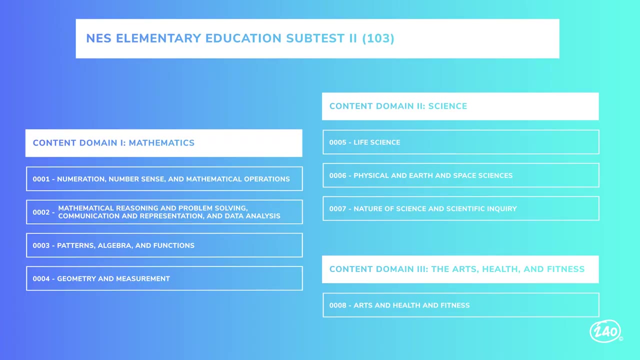 stick around to the end of the video, We just might have some questions about adaptations. Now let's keep cruising through domain two. The next competency is a double whammy. They lumped physical science and earth and space science together, So this covers matter. energy waves, solar system. 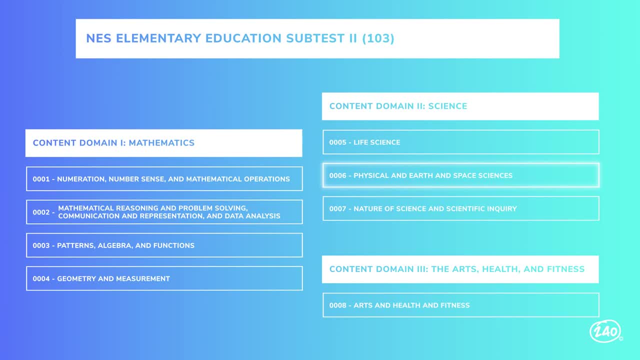 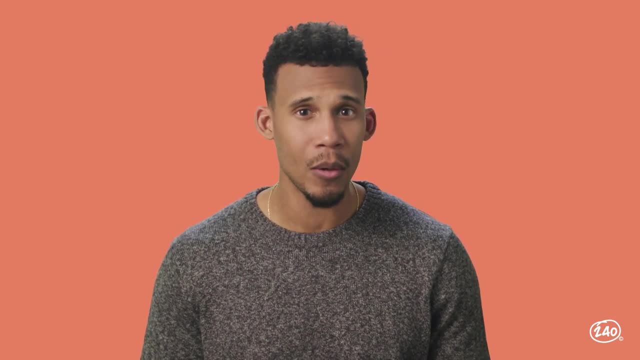 tectonic plates, earth systems and resources available on earth. Whoa Now, while we can't cover every concept on physical science and earth and space, now we'll pick one essential topic that you'll need to know from your exam and zoom in on it. 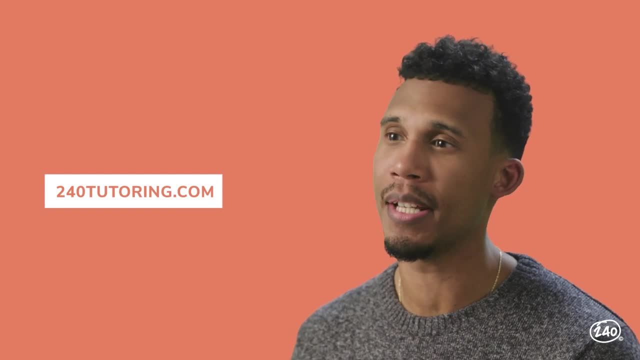 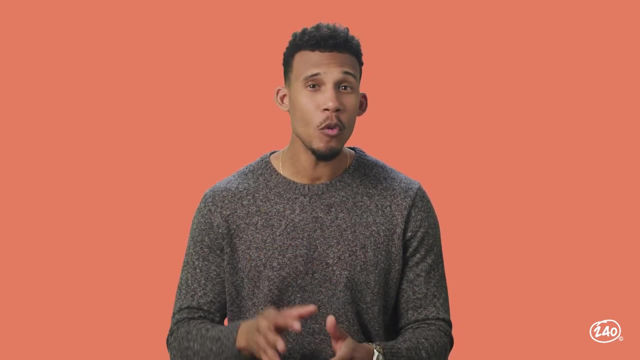 Now remember. if you want more information, you can subscribe to our 240 study guide. We cover all the needs to know so that you can feel confident that you'll pass your exam. Okay, let's get into the movement of the solar system. 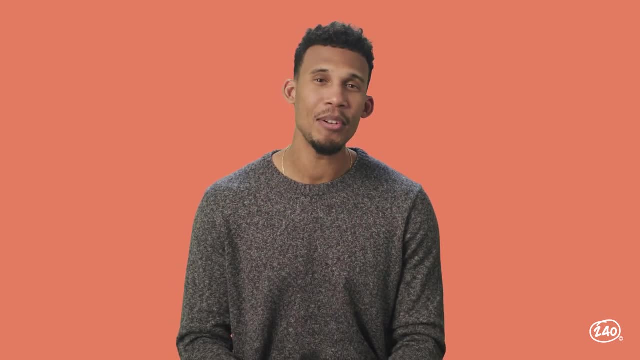 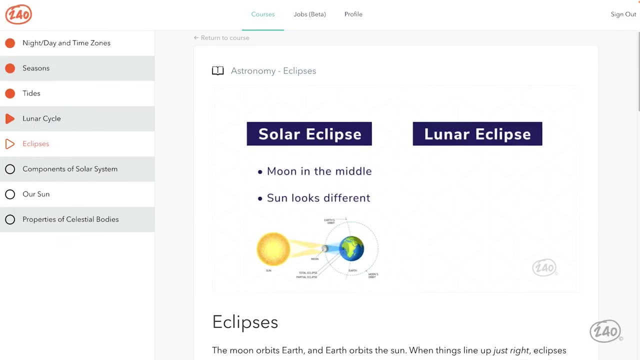 specifically eclipses. I have just the thing to show you. Let's take a peek inside the study guide. Solar eclipses have the moon in the middle and affect the way the sun looks. Think solar equals sun. Lunar eclipses have the earth in the middle. 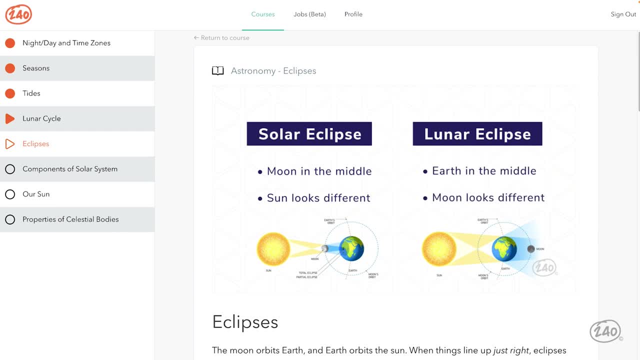 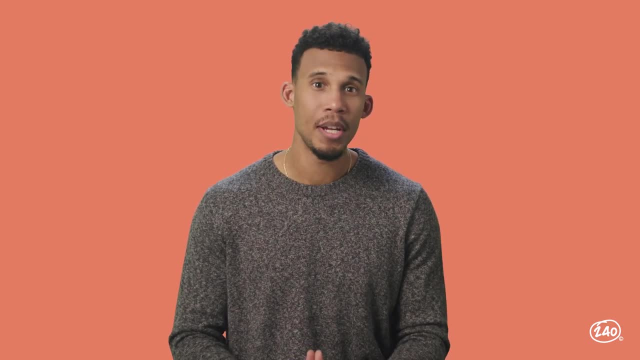 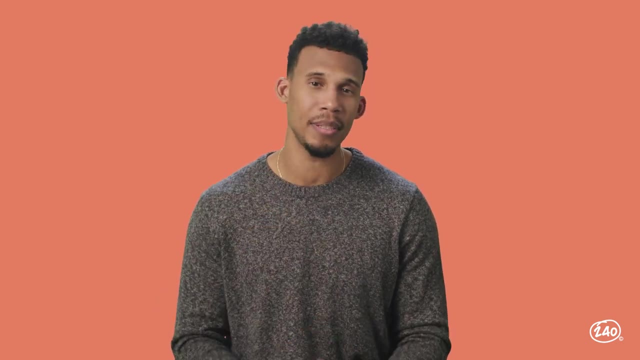 middle and affect the way the moon looks. think lunar equals moon. that preview was just a glance at what we have to offer, and we're so confident in our study guides that we offer a money-back guarantee. now let's wrap up science with our last competency. competency 7 covers the nature of science, which is basically: 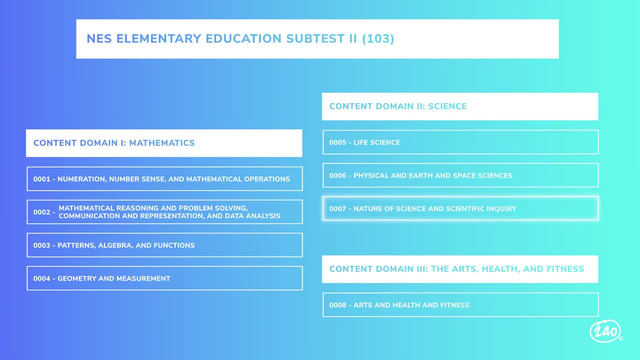 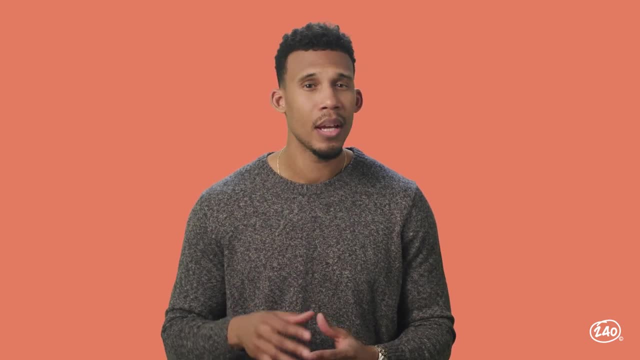 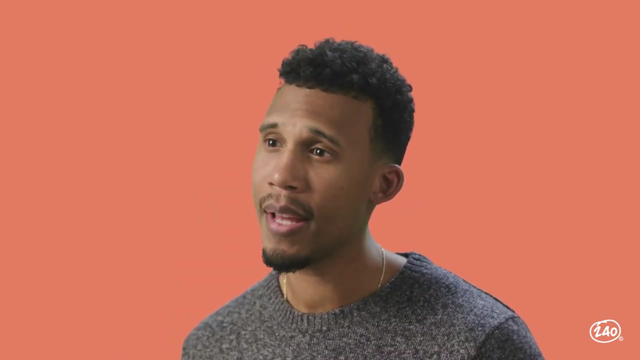 a way of grouping the general scientific practices together. these will apply no matter what branch of science you're studying. you'll need to understand and apply the scientific method collecting and measuring data and how science relates to the other subjects. you'll also need to recognize unifying themes. 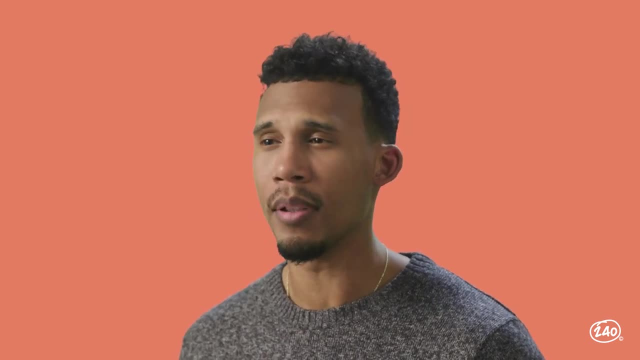 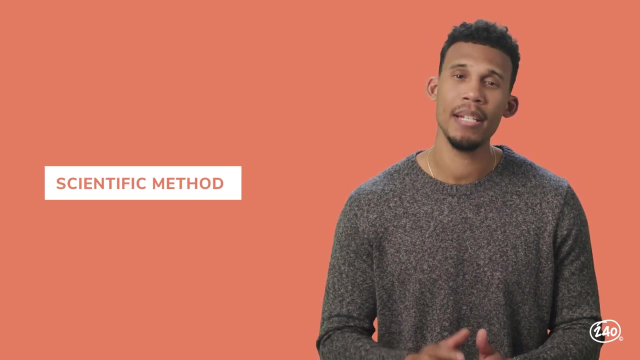 that run between all branches of science, like systems and the relationships between form and function. now I know that sounds like a lot, but the biggest thing to pay attention to is a scientific method need to brush up on those steps a little bit. let's look at a chart from our study guide so we can. 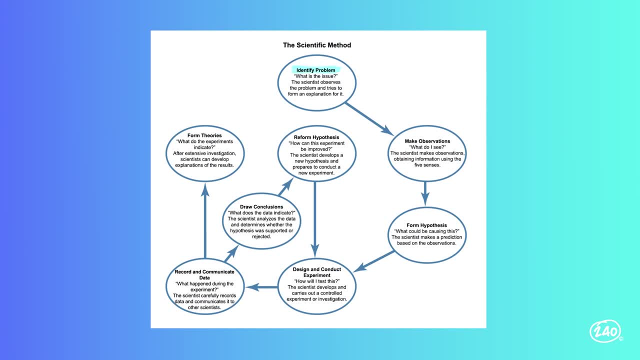 break those down. students start by identifying a problem, then they make observations about the problem, next they form a hypothesis, design and conduct an experiment, record the data they've collected during the experiment and finally they draw conclusions. often scientists use their conclusions to modify their hypothesis and design a whole new experiment. here's another tip you're likely to see. 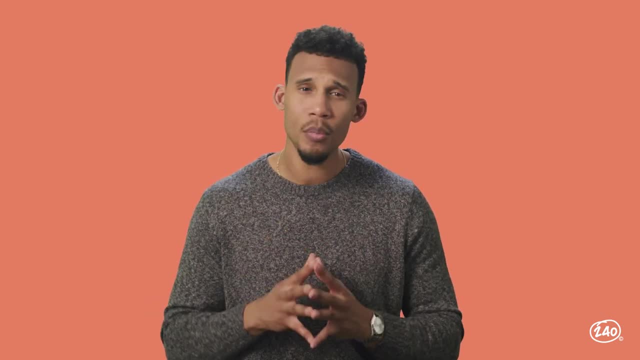 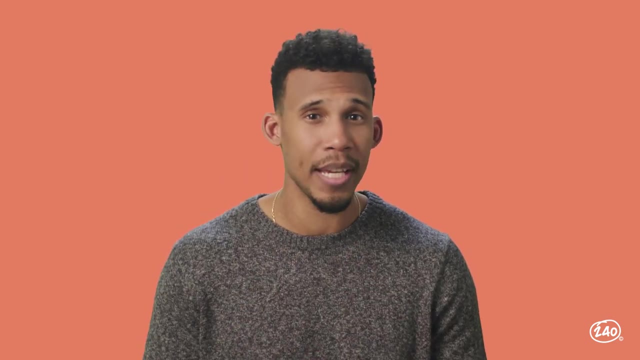 questions on how to best implement each of these steps, not just what they are. so make sure you know how to write a proper hypothesis and set up an experiment. we have plenty more with that came from in the study will do it, but for right now let's dive into the last competency. you're doing great, we're. 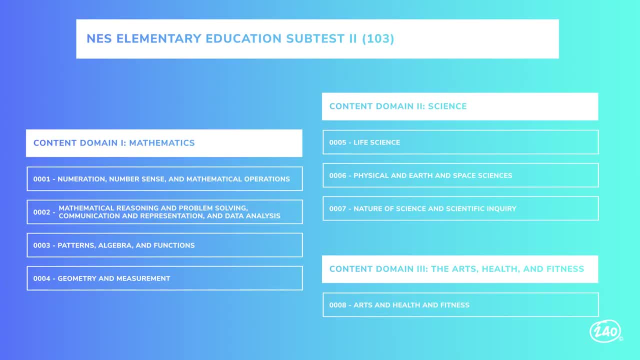 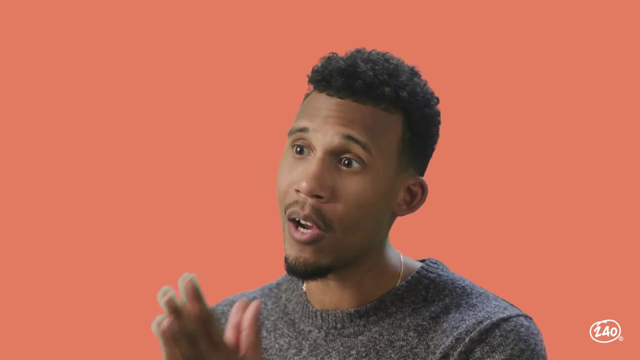 almost to the finish line. we've only got one more domain and one competency left: the arts, health and fitness. you heard me correctly: all of that is shoved into one competency. so, for our part, you need to know the elements associated with music, drama, dance and art and recognize art as communication and self-expression. for pe, you'll need to. 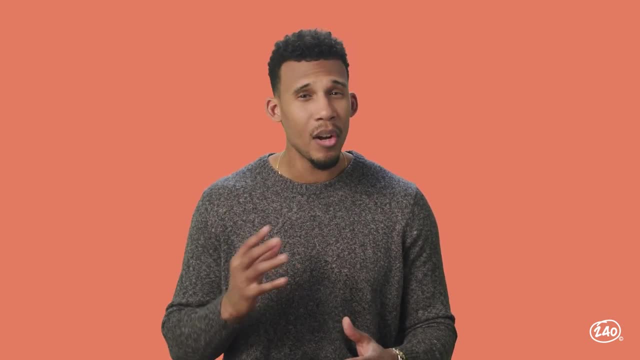 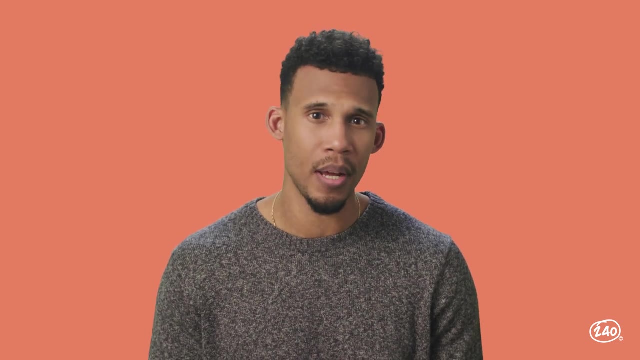 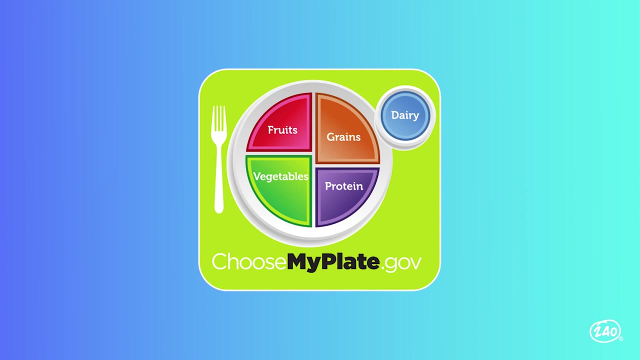 understand the basic structures and functions of the human body and understand how to maintain a physically, mentally and emotionally healthy body. let's focus on health for now. it's important to understand the nutrition needed to maintain a healthy body. the united states fda's current dietary guidelines use the my plate image to show the relative portion sizes of each type of food. 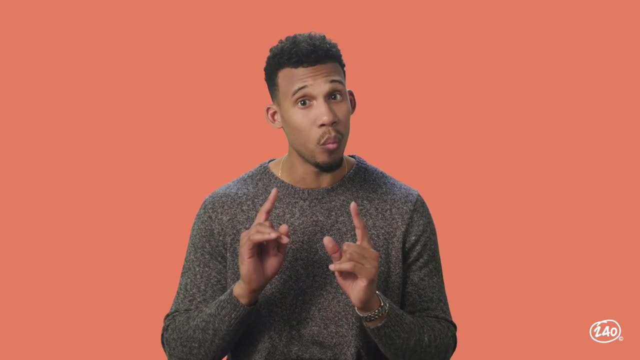 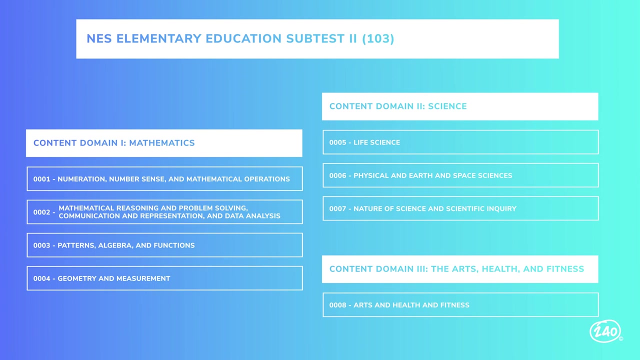 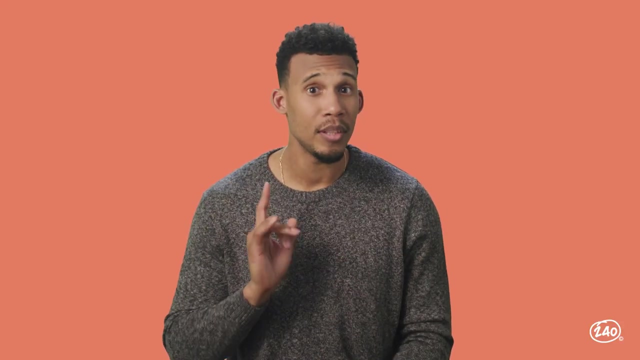 for a balanced meal. but, like i said, that's just one piece of a pretty broad competency. but we've got that all mapped out for you in our study guide. now, that was our last competency and you know what that means. it's question time. let's start at the beginning with domain one. 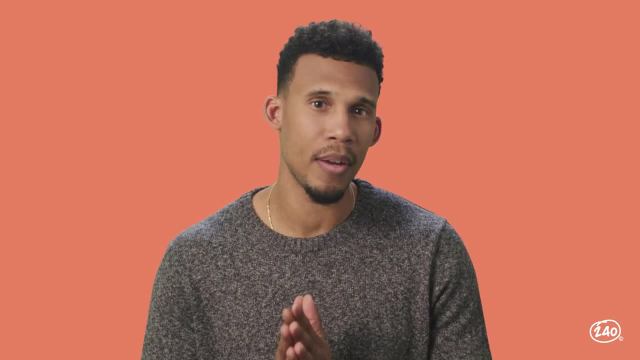 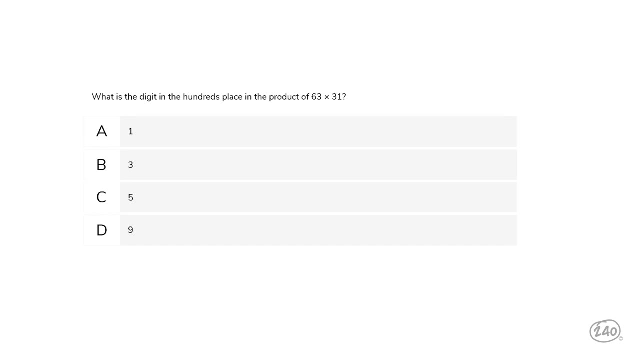 and mathematics. let's take a look at a question about place value. what is the digit in the hundreds place in the product of 63 times 31.. the first step here is to actually do the math. so 63 times 31 equals 1953.. so the answer here is d, the digit that 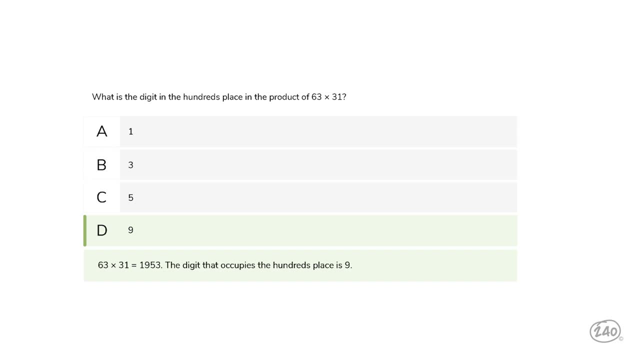 occupies the hundreds place is nine. time for a question about converting between fractions, decimals and percents. what percent is represented by the shaded area of the decimal square? first, we need to figure out what fraction of the figure is shaded. there are 100 total squares and 24 of them are shaded, which will give us a fraction of 24 over 100, which is equal to 24. 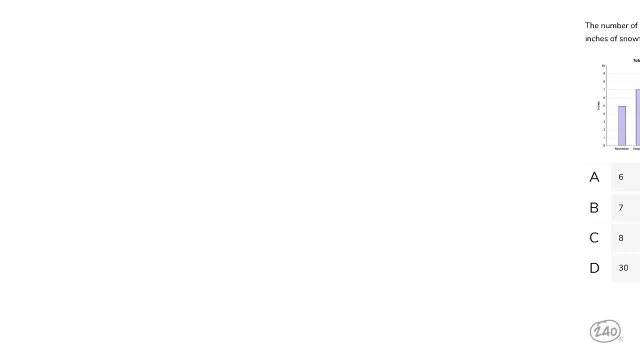 great. let's look at a measure of central tennessee problem. the number of inches of snowfall in selbyville is grabbed in the bar chart below. what is the mean number of inches of snowfall per month from november to march? to find the mean we need to add up all values and then divide by the number of values in the data. 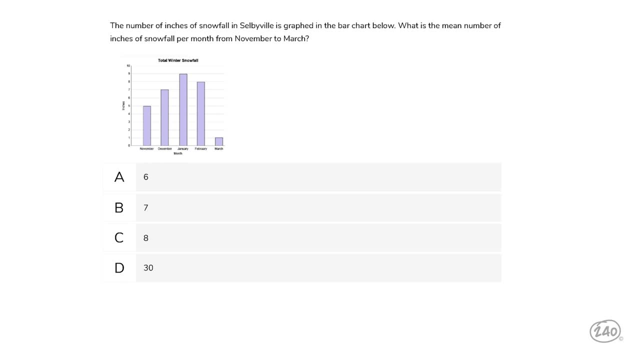 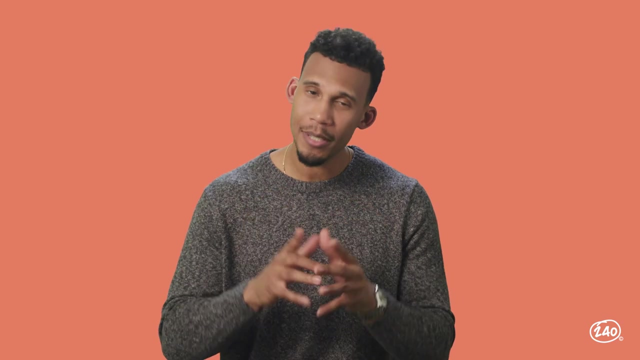 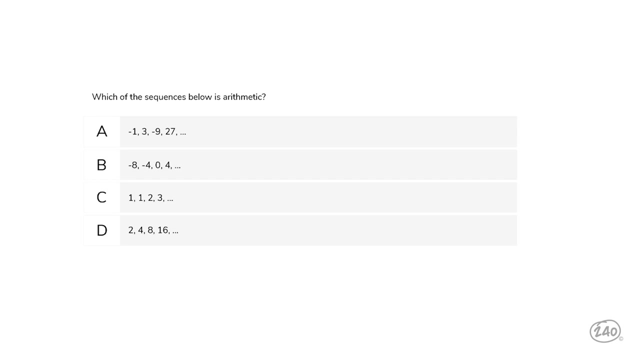 set. so five plus seven plus nine plus eight plus one equals thirty. there are five data points, so thirty divided by five gives us six, so this one is correct. next up in this sequence of questions is a question on sequences. which of the sequences below is arithmetic? an arithmetic sequence is one where the same amount is added or subtracted from each term. 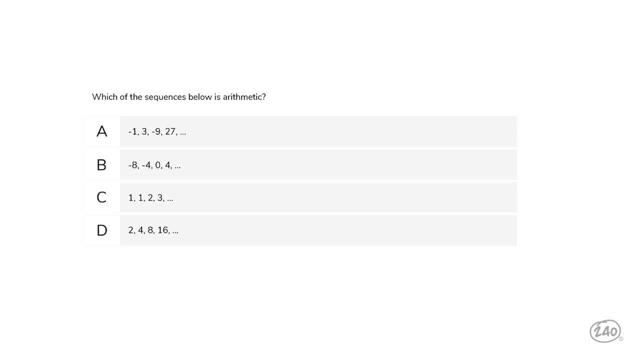 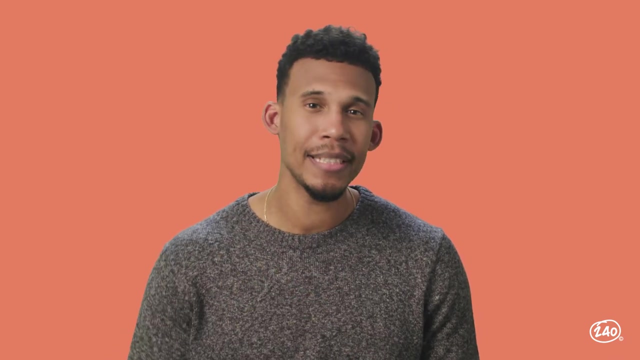 to the next. the only one that meets this criteria is b. this sequence has a constant difference of four, since each term is four more than the preceding term, making it an arithmetic sequence. all right, we're cruising right along. next stop on the math train is similar shapes: a six foot tall. 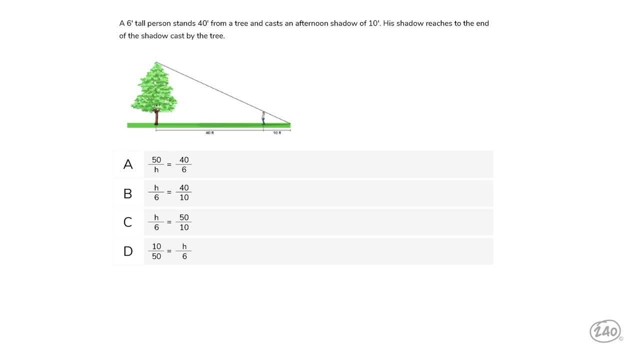 person stands 40 feet from a tree and casts an afternoon shadow of 10 feet, his shadow reaches to the end of the shadow cast by the tree. since we know the length of both shadows, we can build half of our proportion. the man's shadow is 10 feet long and the tree shadow is 40 feet long. 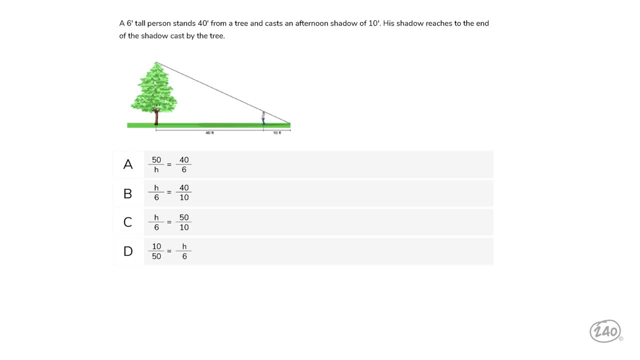 wait, hold up. did you catch my mistake? the problem told us that both shadows end at the same place, so this means that the tree's shadow is 40 feet long and the tree's shadow is 40 feet long, feet long, plus another 10 feet, which gives it 50 feet. okay, so we can use our 10 foot shadow and our 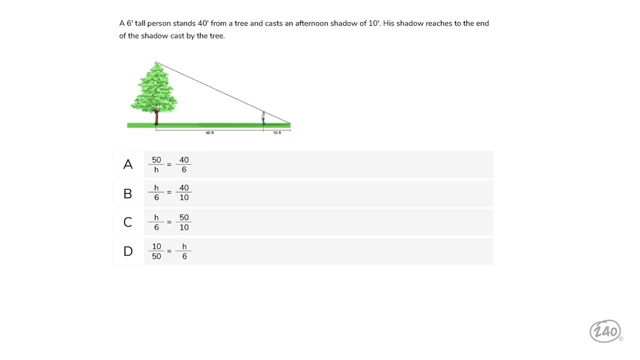 50 foot shadow to build one half of the proportion. so right away, a and b can both be eliminated because they don't have 10 and 50 together in a fraction. next, we know the man is six feet tall, but we don't know the height of the tree, so h? here's where it gets tricky, since the man's 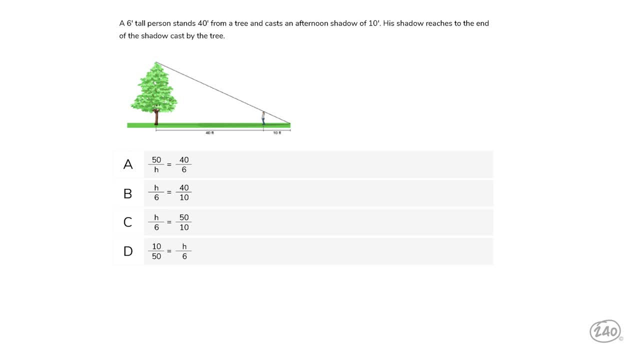 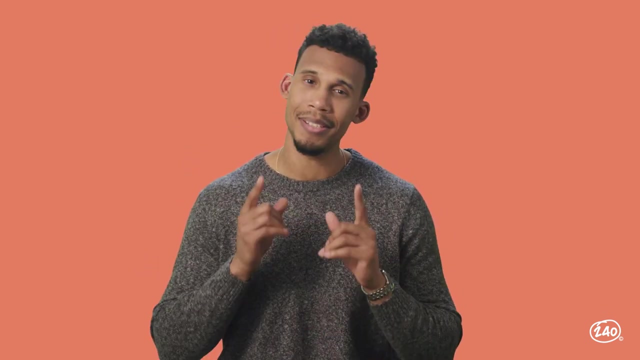 measurements are six feet tall and a 10 foot shadow. those two numbers need to match up, so choice c is the best. six and ten are both denominators of their fractions. domain one done, now let's hop off the math train and switch tracks to science. on to domain two. 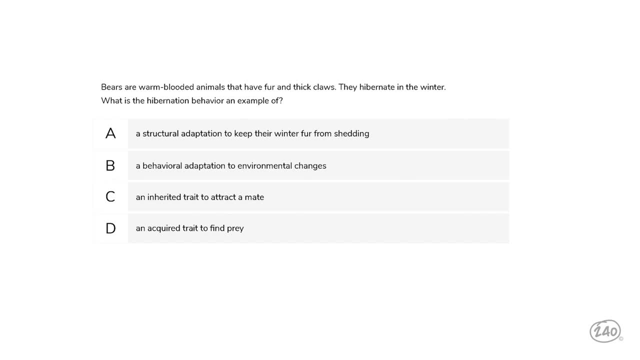 remember when we talked about adaptations. bears are warm-blooded animals that have fur and thick claws. they also hibernate in the winter. what is the hibernation behavior? an example of this is definitely an adaptation, and, since we're dealing with something that the animal does, 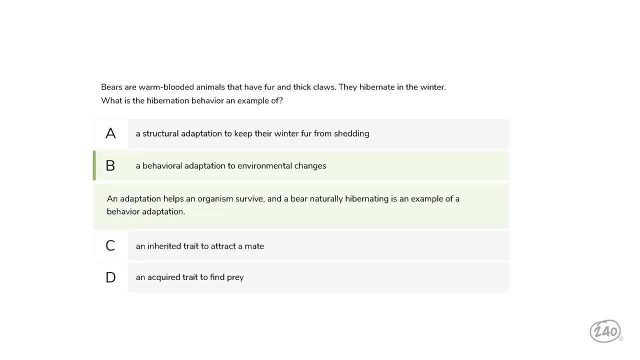 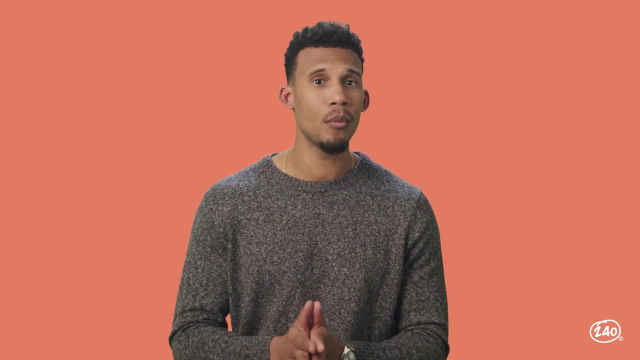 instead of a trait the animal has, b is best. an adaptation helps an organism survive and a bear naturally hibernating is an example of a behavior adaptation. now we're in the combo of physical and ecological and earth science. i know we talked about eclipses before, but how about i show you? 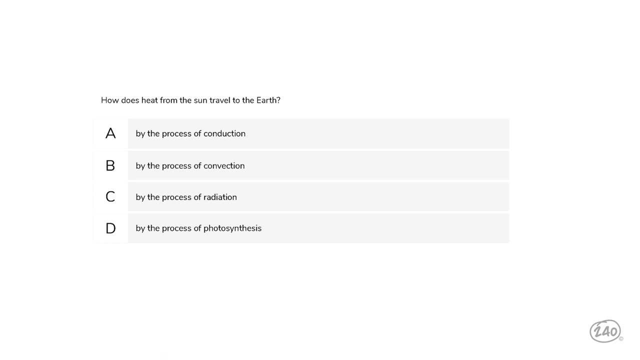 one that brings in physical science too. oh, conduction, convection, and radiation comes up a lot here. how does heat from the sun travel to the earth? now, right away, we can cross off photosynthesis. that's a process done by plants to create sugar that can be used as energy. the sun warms the planet. 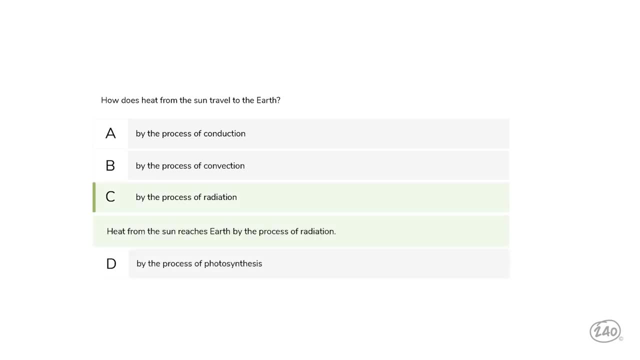 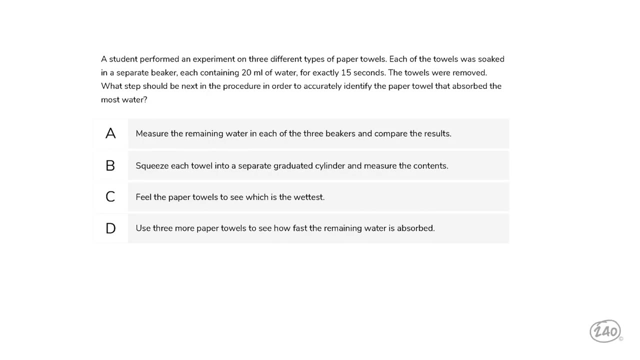 by sending heat in the form of electromagnetic waves. This means radiation is the best answer. All right, one more from the science competency, The scientific method. A student performed an experiment on three different types of paper towels. Each of the towels was soaked in a separate beaker. 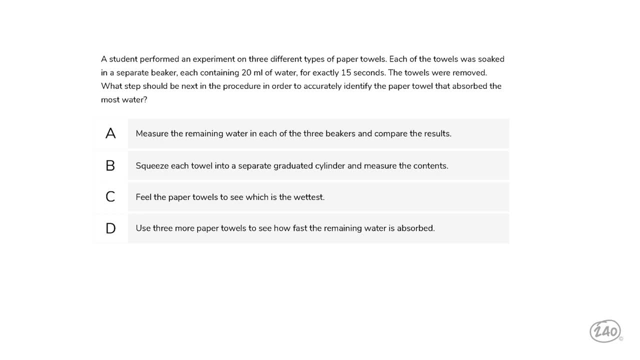 each containing 20 milliliters of water. for exactly 15 seconds, The towels were removed. What steps should be next in the procedure in order to accurately identify the paper towel that absorbed the most water? There is only one answer here that allows us to get a measurable difference. 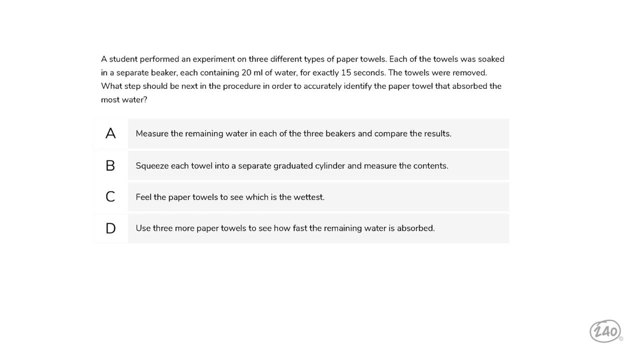 in our paper towels, which is super important whenever you're conducting an experiment. Choice A is correct. To accurately compare the paper towel absorption, the amount of water remaining in each of the beakers must be measured and compared after removing the soaking paper towels.